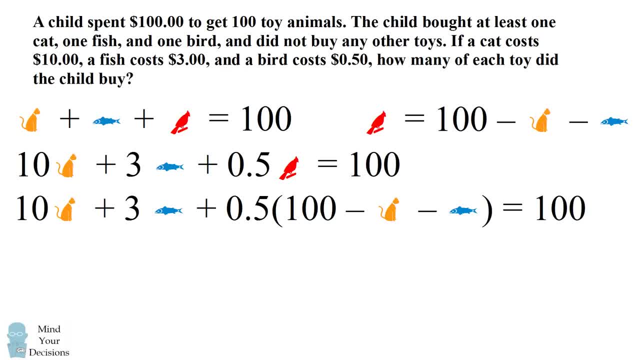 We can substitute that into the second equation. We'll now simplify this and then we'll simplify it further. We end up that 19 times the number of cats plus 5 times the number of fish is equal to 100.. Let's continue from this equation. 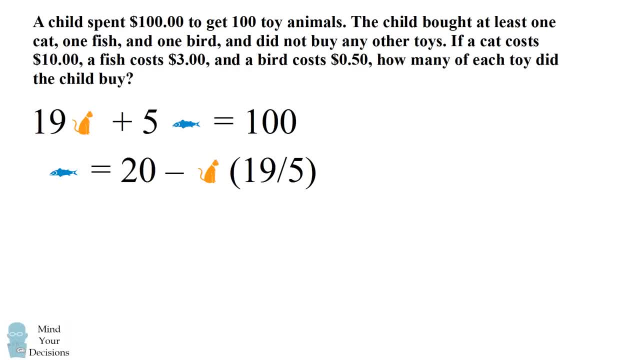 We'll solve for the number of fish We have. the number of fish is equal to 20, minus the number of cats, times 19 over 5.. This will be the key equation to deduce the answer. The variable cats is being multiplied by 19 over 5.. 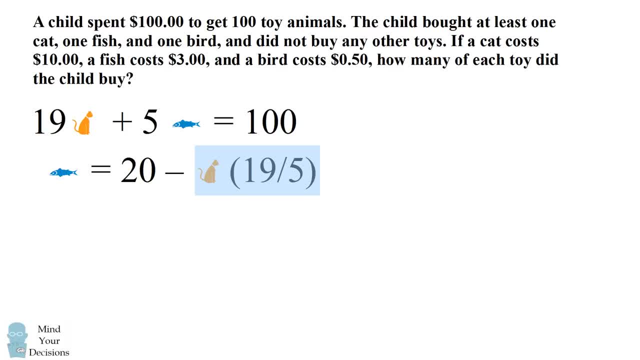 Now we need the number of fish to be a whole number, and we know that the number of cats is also a whole number. This means the number of cats has to be a multiple of 5, so that the number of fish is a whole number. 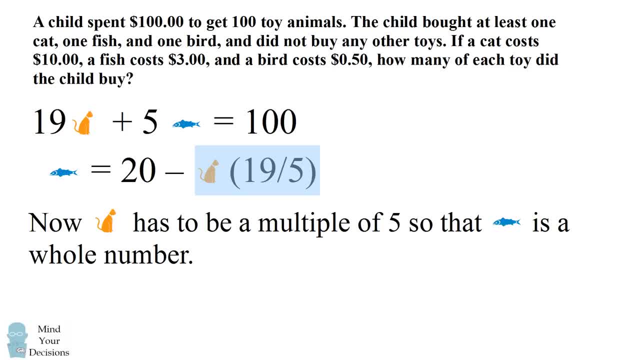 Furthermore, we need the number of fish to be a number that's greater than 0. We're taking 20 minus the number of cats, times 19 over 5. So we can figure out that the number of cats has to be less than 100 over 19,, which is the number of cats. 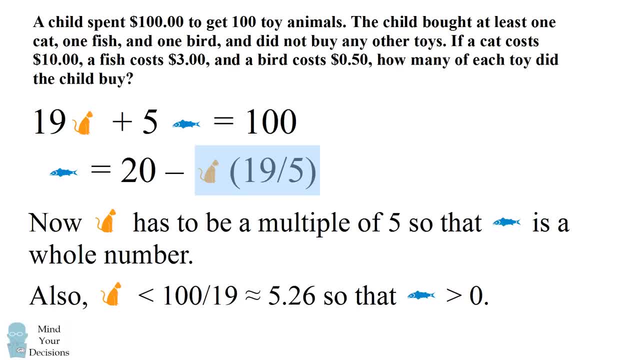 Or approximately 5.26, so that the number of fish is greater than 0.. So we need a multiple of 5. that's less than about 5.26, and we know that the number of cats is also greater than 0.. 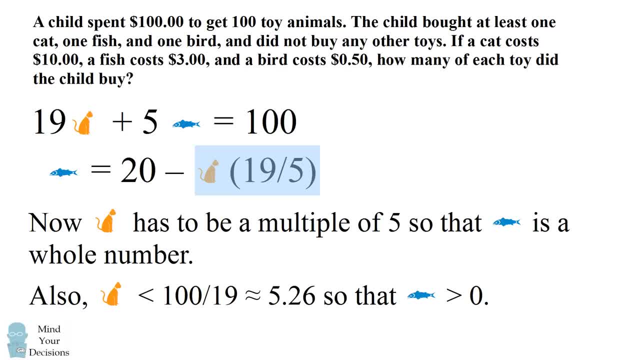 So what number is a multiple of 5 that's greater than 0 but less than 5.26?? There's only one possibility, which is that the number of cats is equal to 5.. So we've uniquely solved for the number of cats and we can substitute that value to get that, the number of fish has to equal 1.. 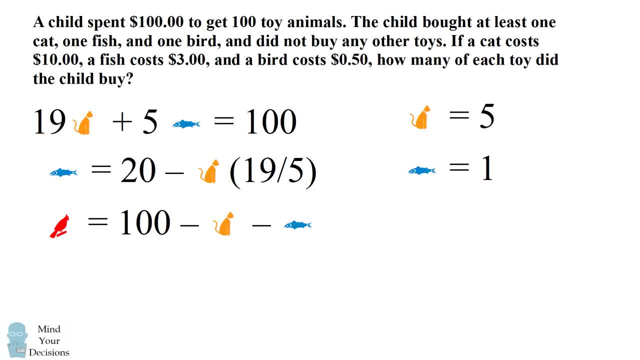 We now need to figure out the number of birds, but we know the total number of animals is equal to 100. So we can then say that the number of birds is equal to 94. And this is the unique solution to this problem. 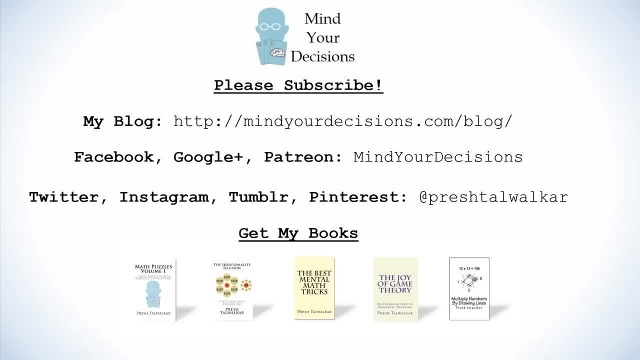 Did you figure it out? Thanks for watching this video. Please subscribe to my channel. I make videos on math and game theory. You can catch me on my blog Mind Your Decisions, which you can follow on Facebook, Google+ and Patreon.